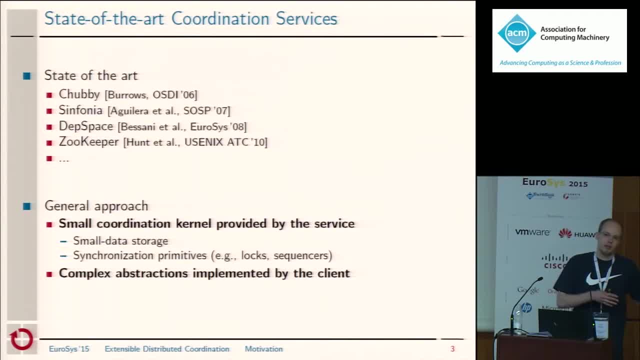 share this common approach of not directly implementing all kinds of coordination mechanisms, but instead to provide a small set of very generic functions, which is also called a coordination kernel: Maybe some methods for small data storage, maybe one or two small synchronization primitives, So to have this small set of functions which would then allow 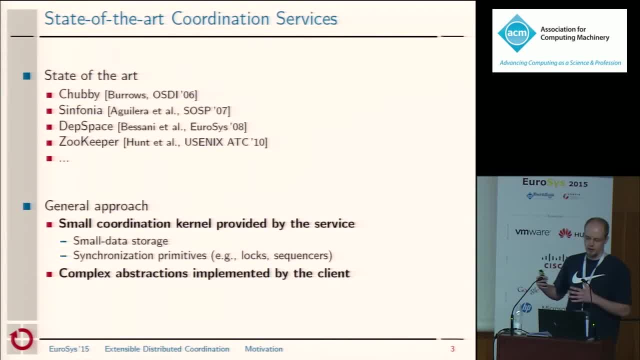 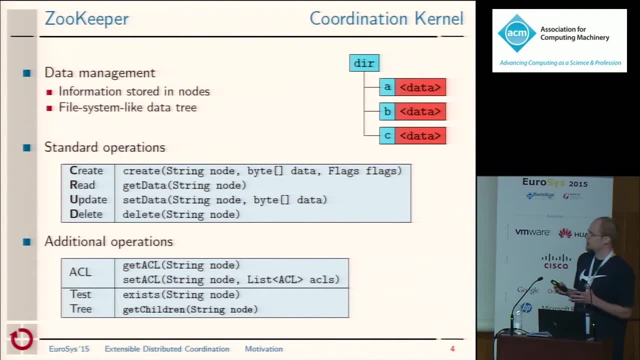 a client to build more complex abstractions at the client by using these functions. Now let's take a look at how this works in ZooKeeper. ZooKeeper stores data in nodes in a file system like DataTree and provides some generic functions. So create those nodes. 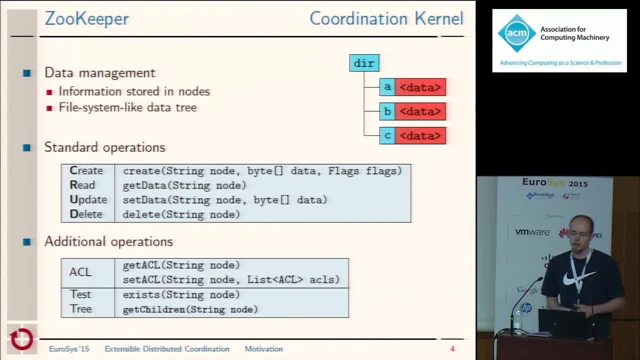 set the data of those nodes, read the data from those nodes, delete those nodes. so you have your typical CRUD operations And in addition to that there's only a small set of additional functions to manage access control, to check whether a node exists or not, And 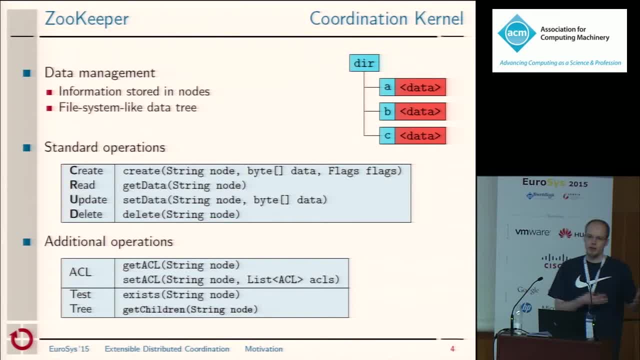 there's this getChildren call which, for example, allows you to retrieve the names of child nodes. So, for example, if you called this getChildren on this dear node, you would get A, B and C. So, as I said, a small set of functions, very generic. Let's take a look at how you build. 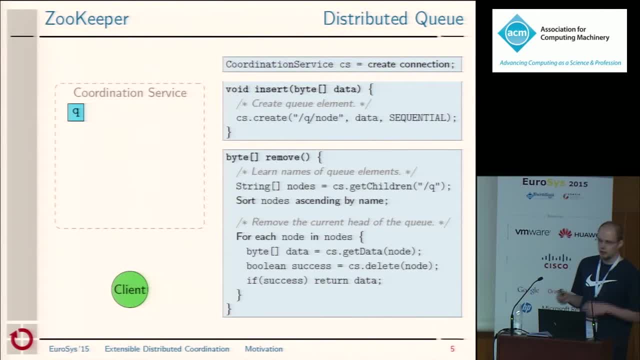 more common actions, More complex abstractions on top of that, using the distributed queue as an example. So the implementation of the distributed queue here has two functions: an insert function that allows a client to add an element to the queue, and a remove operation which allows 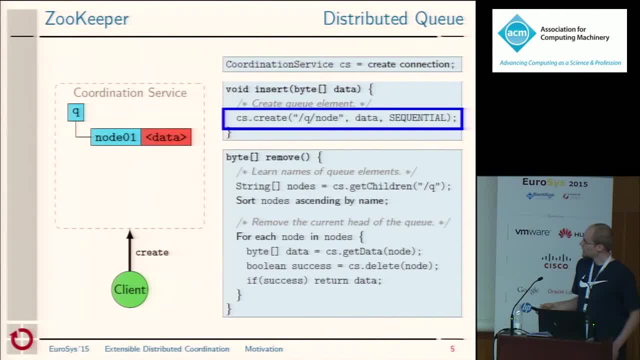 a client to remove the current head element from the queue. So, as we see here, the insert method is rather simple. All it does is it creates a node in the coordination service, assigns the data to it. Now, what the sequential flag here does? 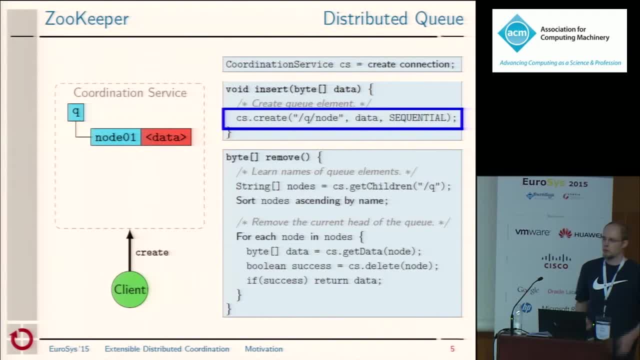 is, it tells ZooKeeper to not only create the node with a specific name, but to add a sequence number which is automatically increased to the node name. So the first time we call this insert method, it will create a node 1.. And if we call this multiple times, 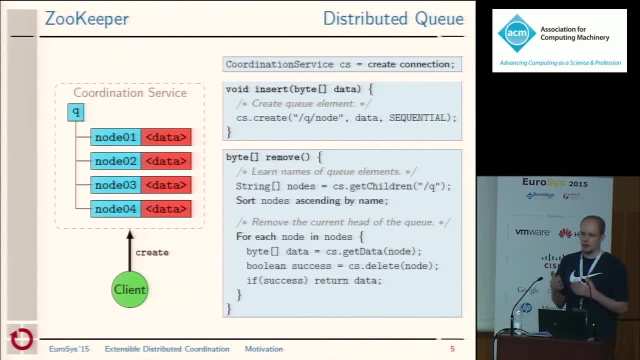 we end up with nodes 1 through 4,, for example, The sequence number automatically increases. We've seen the insert method is rather straightforward: only a single remote call. The complexity is part of the remove operation. To be able to remove the head element of the queue, what the client first has to do is 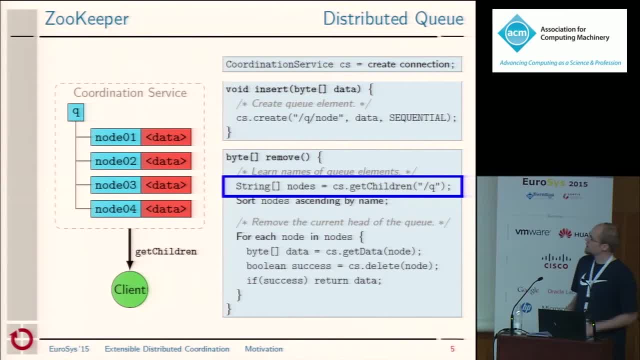 it has to identify this element. So the way this works in ZooKeeper is: the client takes this getChildren call in order to learn all the node names and, using the sequence number encoded in these names, the client is able to detect the head of the queue, which is 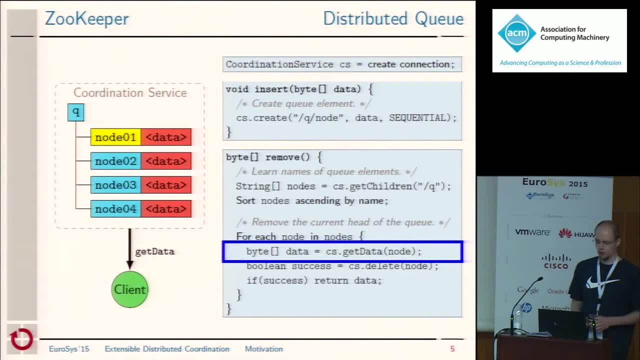 the node with the lowest sequence number, So in this case it is node 1.. So having found this head element, the client is able to get the data. So we start by calling the method on the coronation service and then finally to remove the head. 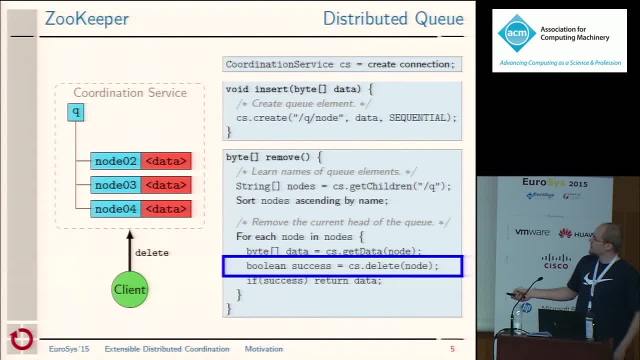 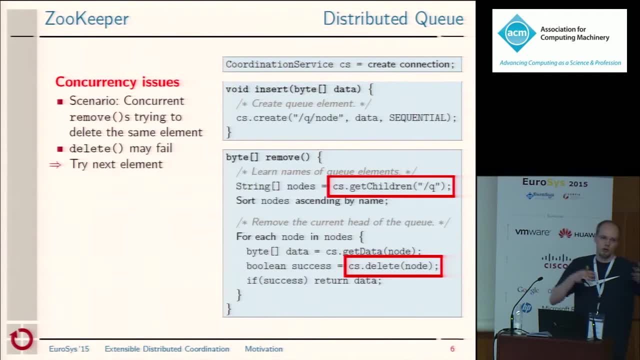 element by using delete. So we see that surrounding the last two statements, there's this for loop, and this is required because there may be scenarios where two or more clients can call the remove function concurrently, And there may be scenarios in which two clients call this getChildren concurrently, which 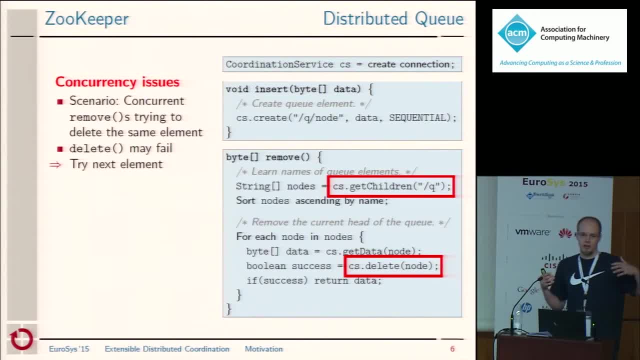 means they download this function and then return it to the client. So this is a really the same list of nodes, which means they identify the same node as current head element, which means they try to delete the same node. So in these cases, ZooKeeper ensures that only one of the 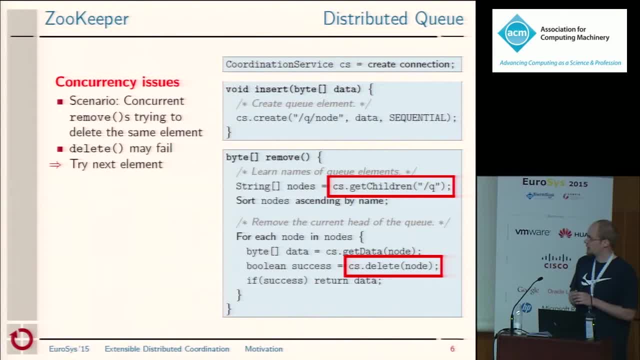 clients will actually be successful. So this is the client which gets a confirmation from ZooKeeper: okay, the node is deleted and this is the client which is actually able to successfully complete its remove operation. The other client will get an exception from ZooKeeper saying the: 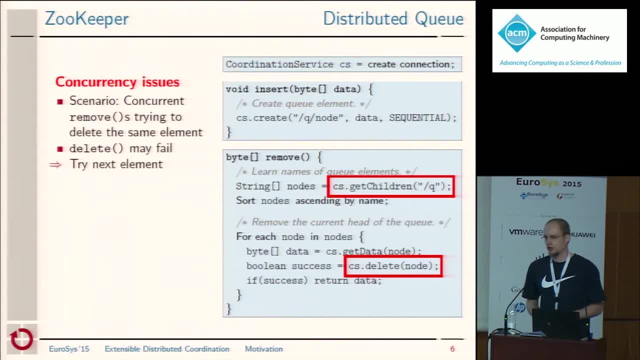 node you're trying to delete does no longer exist and this is a signal to the client to enter this for loop once more and to try with the next element. So we've seen a first drawback of this kind of implementation. There may be retries, multiple retries, until we're actually successful. 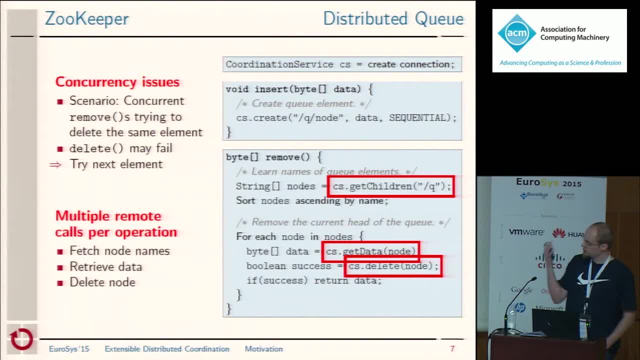 to remove an element. Another drawback of this solution can be identified just by looking at the code. Even in the best case, we need three remote calls from the client to the server. So we need three remote calls from the client to the server. So we need three remote calls. 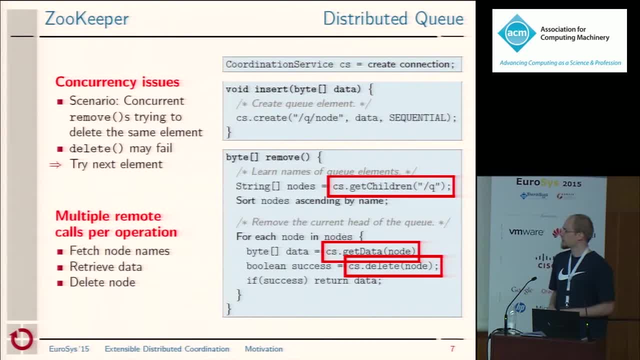 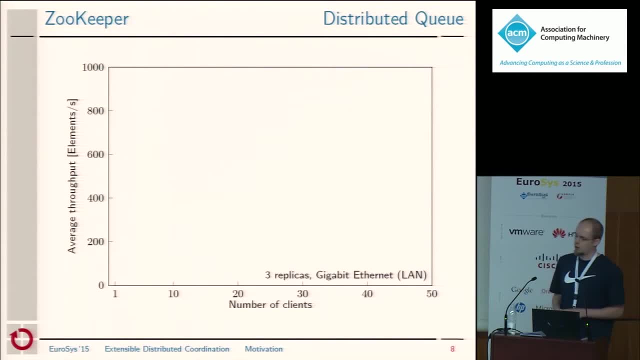 from the client to the server in order to remove even a single element, which is not optimal in terms of latency. Now let's take a look at how this translates. to throughput What we did was we ran an experiment where we had clients continuously adding an element to the queue, removing an 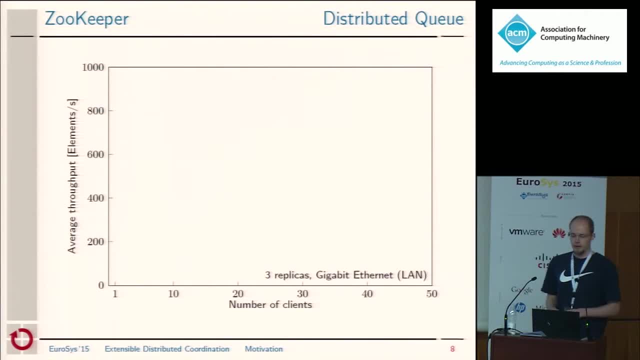 element from the queue, adding an element from the queue, removing and so on. And here's the results in terms of throughput. So higher is better. For a single client, the queue achieves a throughput of a little over 200 elements per second. 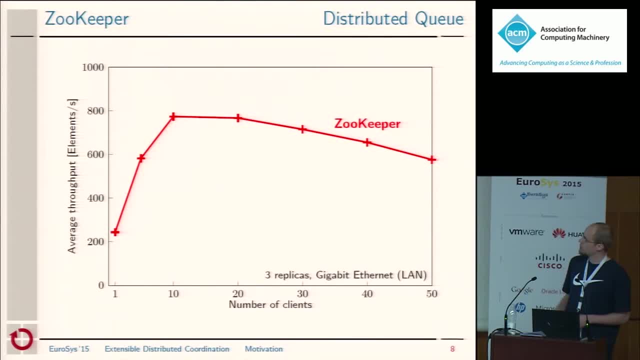 The throughput increases with more clients to just under 800 elements per second. but then, adding more clients, it decreases, And the reason for that is with more and more clients we have more and more concurrently, The success rate of the delete operation will drop dramatically, so reaching 2%. 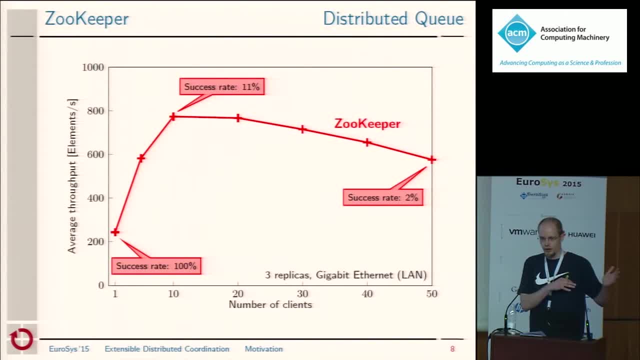 for 50 clients, And this is why the throughput drops. The problem here is the coordination service. in this case, ZooKeeper still has to perform all those operations, but fewer and fewer clients actually are able to make progress And again, this is a 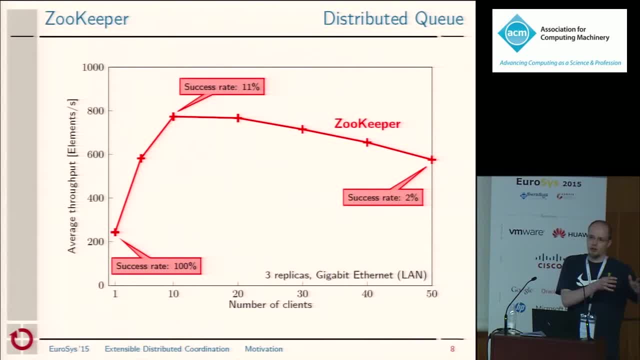 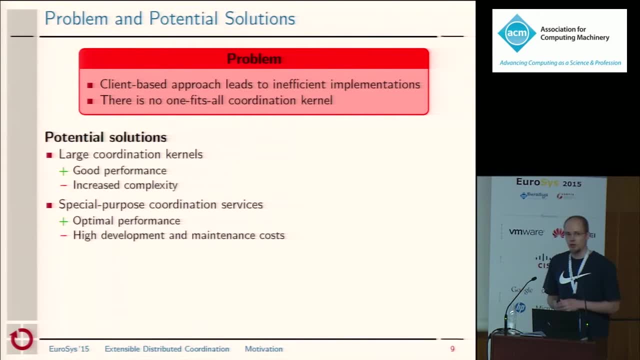 consequence of this general approach to have this small set of generic functions and to build more complex abstractions at the client. Now we further investigated this problem. We looked at different coordination mechanisms, We looked at different coordination services and it turns out this is: 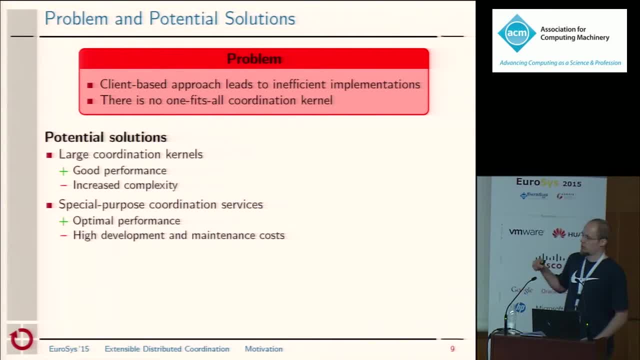 not a problem specific to distributed queues, and it is not a problem specific to ZooKeeper. In contrast, it is a problem of the fact that there is no small one-fit-all coordination kernel that would allow several or all kinds of coordination mechanisms to be efficiently implemented at the client. 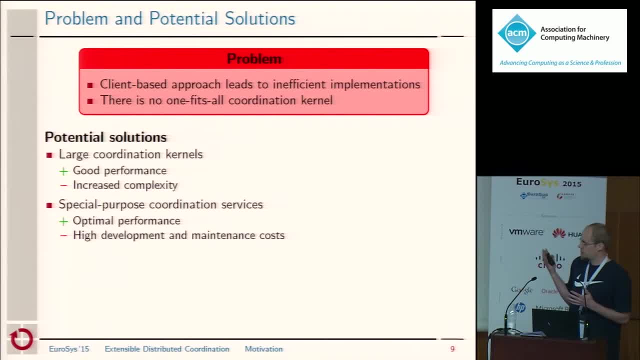 Now what can we do about it? There are basically two possible solutions. First, what we can do is we can add new functions to the kernel. For example, if we had a queue remove operation in ZooKeeper, we probably would be able to. 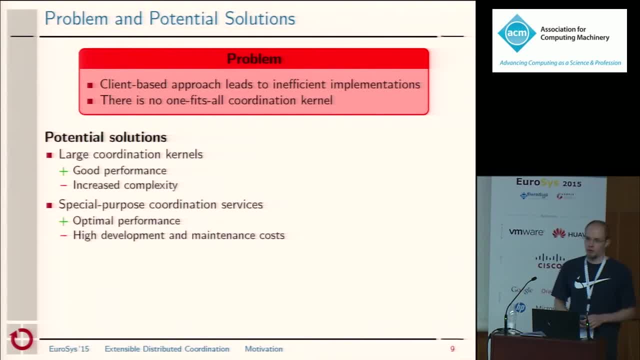 implement this in a kind of a more simple way. So, for example, if we had a queue remove operation in ZooKeeper, we probably would be able to implement this in a kind of a Or in the way that we achieve good performance. But the problem is: with more and more functions the kernel gets more complex, makes it harder to maintain. 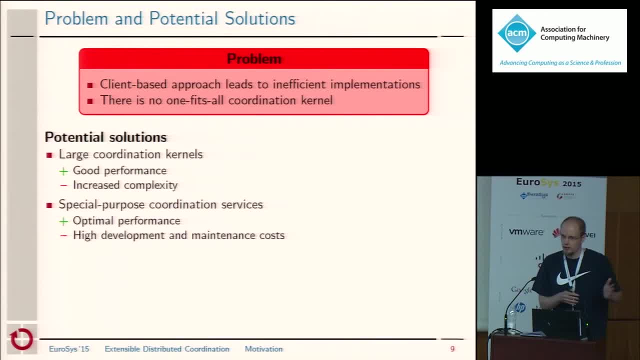 So we actually don't want to do that. another alternative solution would be to have dedicated correlation services for each for all kinds of correlation mechanisms. This would have the benefit of being able to optimize for certain data structures. So, for example, we could optimize a correlation service for 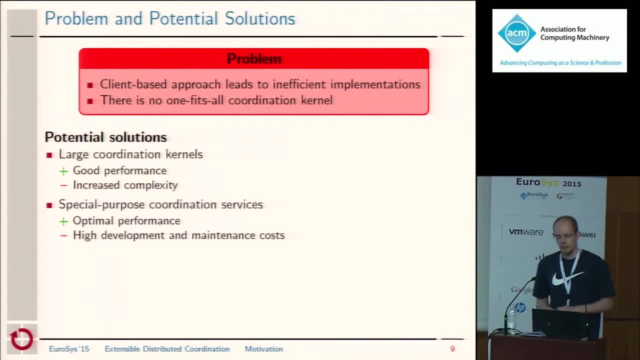 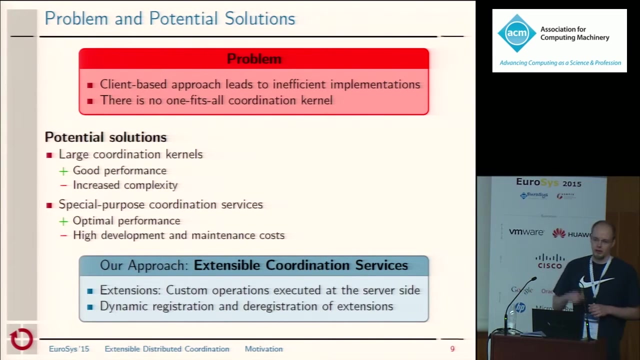 Distributed queues. But the downside here would be, instead of having a single correlation service in the data center, We would now end up with multiple correlation services. so this also makes it harder to maintain and There are high development costs. So our approach is different. What we did was we made the correlation service extensible, and by that we mean a client is able to write custom operations. 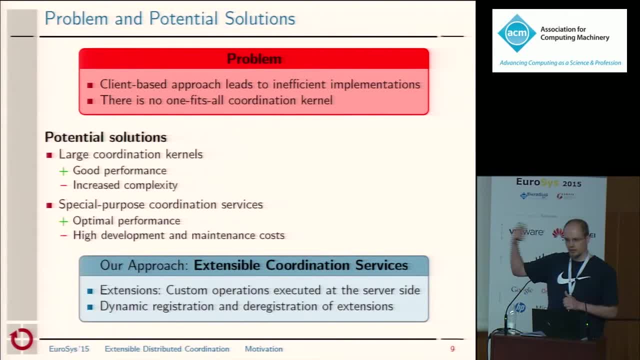 To register them at the service, To invoke them as long as it needs them and after the client doesn't know, when the client does not need them any longer, the the custom operations are removed and This way we would get the best of both worlds. We would still have a small coordination kernel, but we would achieve- or we will achieve- good performance due to executing. 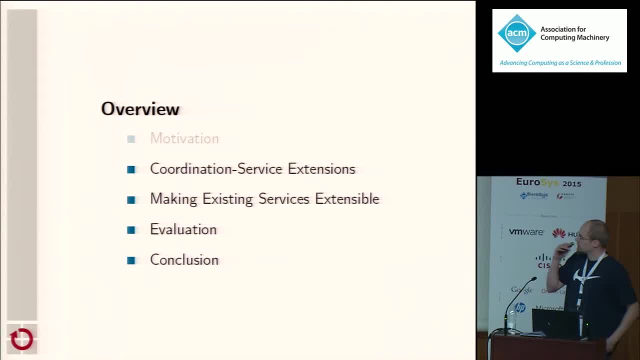 most of the stuff at the server. So now there's some my talk. I'm first going to talk a little bit more about what our correlation service extensions show, an example of how such an extension might look like. I Will go into a little bit more into detail on how to make existing correlation services extensible and 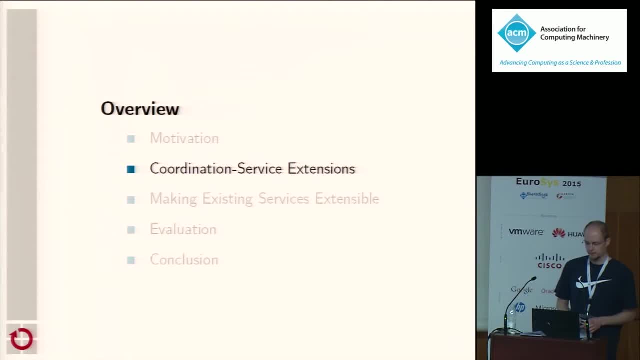 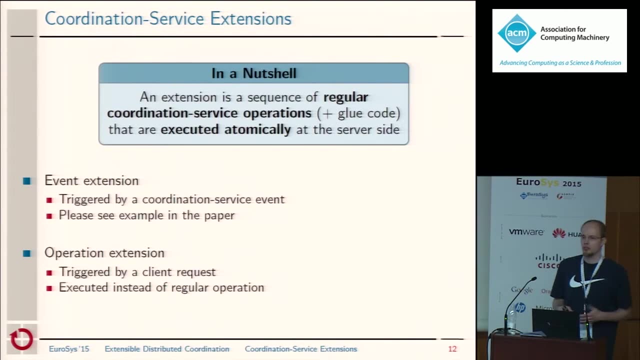 At the end I will briefly present some evaluation results. Now. in a nutshell, what is a correlation service extension? It is a sequence of regular correlation service Operations plus a little bit of glue code that are executed atomically at the server side. Now what is important here is that an extension is not a means to run arbitrary code at all. 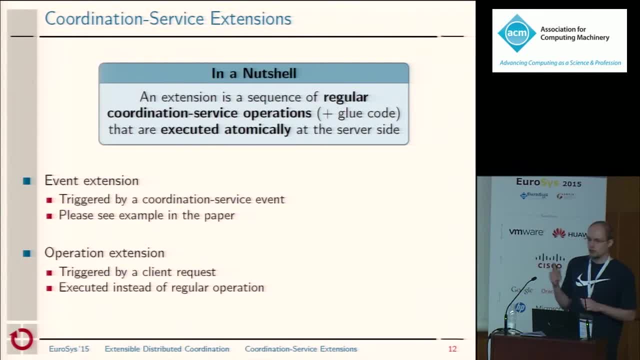 The service at the server side. so we want an extension to be a composition of correlation service operations. Extensions come into one of two flavors: event extensions and operation extensions. and the next, event extension, is a Means to customize the reaction of the correlation service to certain events. I won't go into detail. 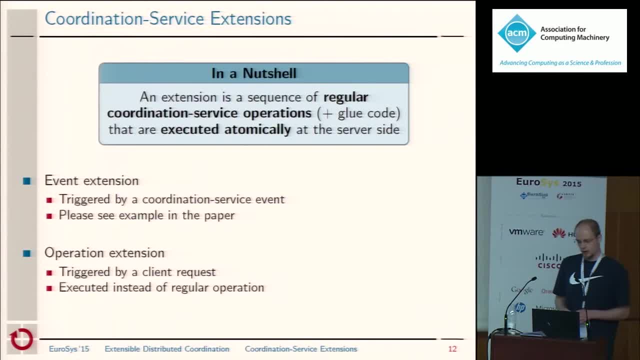 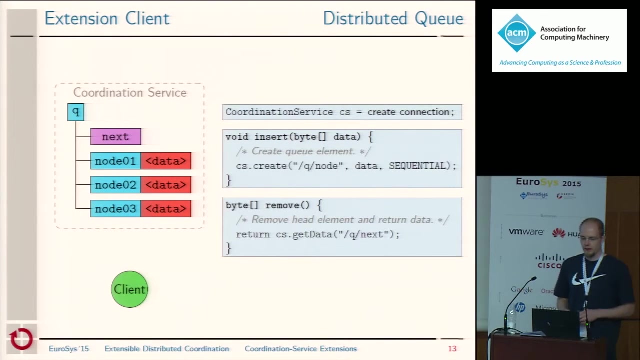 for this kind of extension. So please refer to the paper for an example. I will focus on falling on the other type of extension, the operation extension, Which is triggered by a client request and which basically overrides the regular operation of the correlation service for a certain node. So using such an operation extension we, for example, can refine the distributed queue implementation. now, before we actually look at the extension, 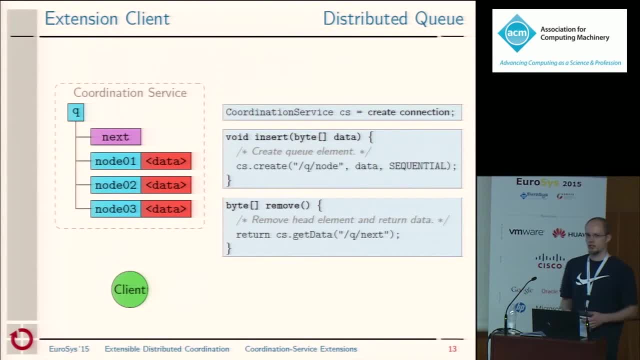 Let's take first a look at how a client uses such an extension. As we see here, we have the exact same Methods as before. in fact, the insert method has not changed at all. It is exactly the same as in the regular implementation. However, the remove operation has changed dramatically. 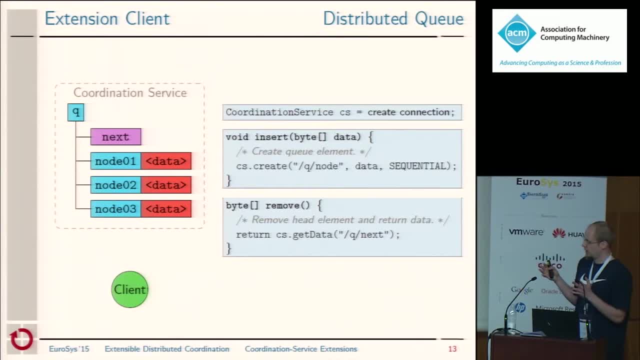 So, instead of doing all those steps, all the client does in this case is to invoke the get data operation on a call, a node slash, slash, queue, slash next, and when this operation returns, the client will have the data and The element will. the current head element of the queue will have been removed. 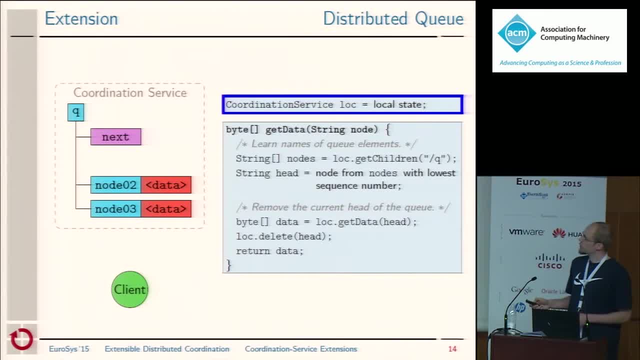 So how does this work at the server? The first difference we notice is that an extension, in contrast to a client, is able to Locally access the correlation service state. so we don't need Remote calls anymore. all stay a calls to the state from an extension or local. 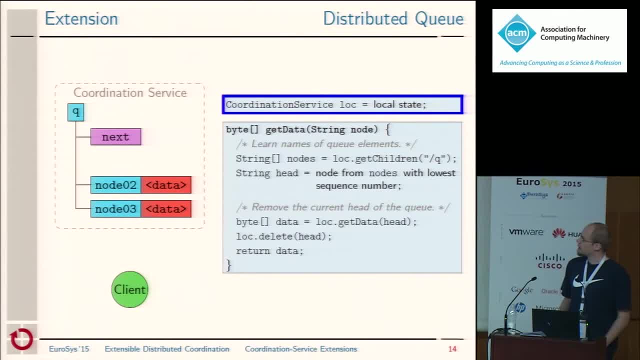 So that's good in terms of performance. now, in this case, as I said, the extension is Triggered when someone calls get data on this node next, And what the extension does is it performs basically the same steps as the client has done in the regular implementation, And this makes it easy for programmers who know how to write extension. 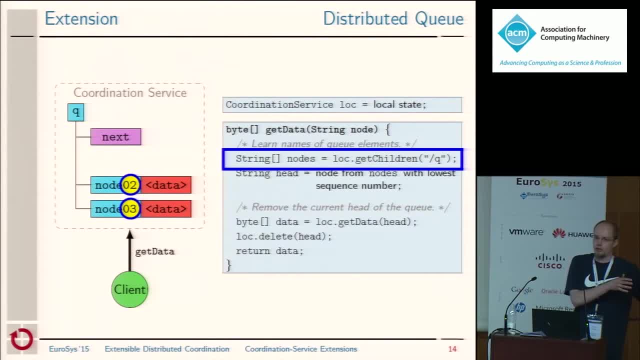 Know how to write abstractions for a certain coordination service to also implement Extensions for this very same correlation service. So in this case, what the extension does is that tries to identify the first element in the queue By looking at the sequence numbers, and as soon as the extension has found this, it gets the data. 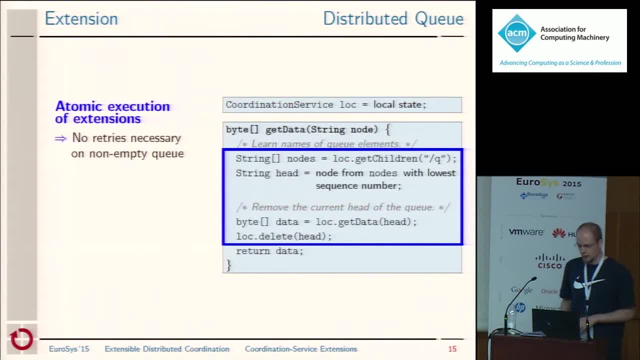 deletes the node and returns the data. The big difference is we don't need a for loop because all those steps are executed atomically, so there are no retries necessary if We have elements in the queue. So that's a good thing. another benefit also mentioned: the client only needs a single remote call to actually 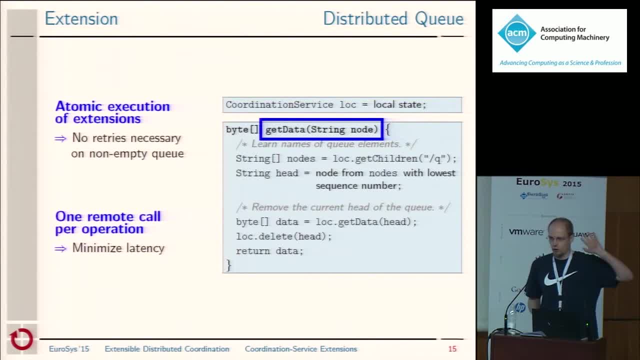 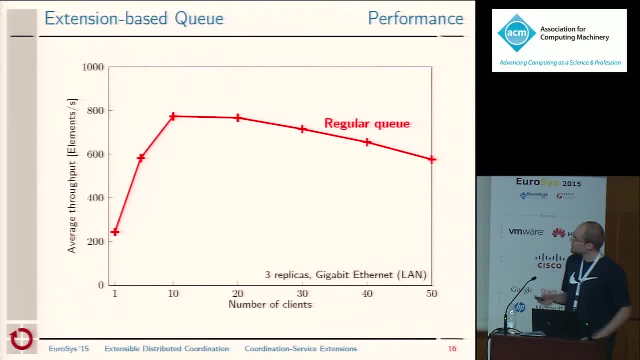 Remove an element, So no more three or four or five or more remote calls necessary. So what's the impact on throughput? This is the results, the zookeeper result of the regular, of the regular queue. The first thing we learned is that we need a bigger scale. 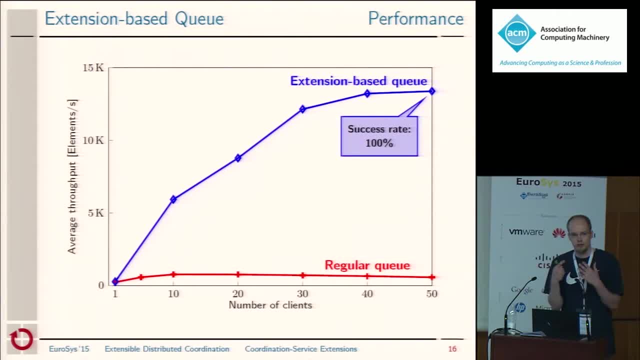 Because, due to the fact that there are no retries, due to the fact that remove operations on a non-MTQ always succeed, We have a success rate of 100% for the roof operations and this allows The extension based queue implementation to achieve above 14,000. 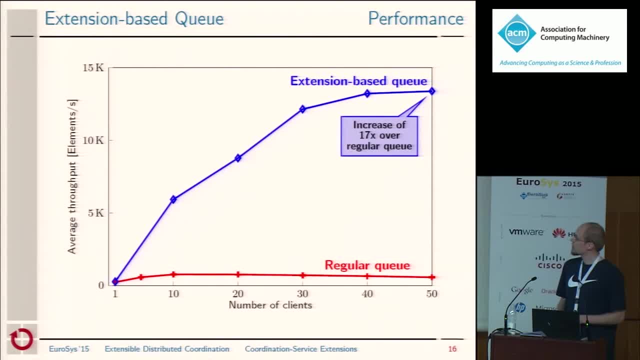 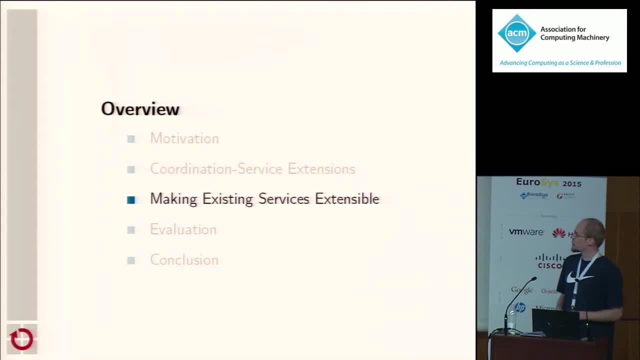 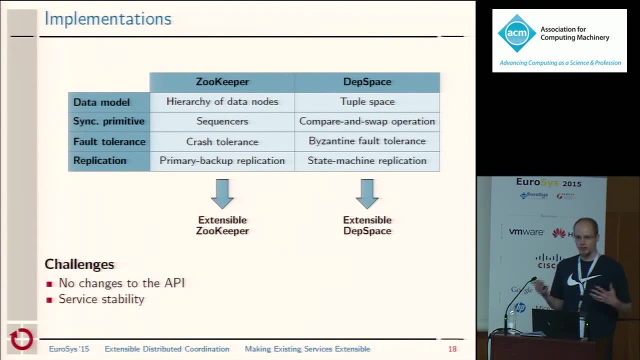 elements per second, Which is a factor faster or more throughput by a factor of 17. Now, if you weren't on implementation, what we did was we took two existing correlation services, zookeeper and depth space, Which are quite different and that they use different data models. They provide different synchronization primitives. 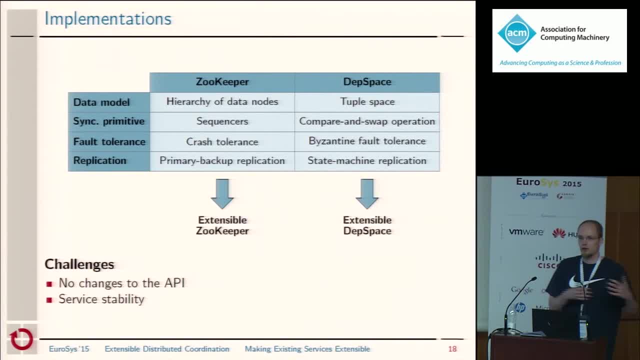 They offer different fault tolerance guarantees. one is crash-tolerant, one is by some time fault-tolerant. They use entirely different replication approaches: a primary backup replication in zookeeper, slave machine, replication by some time fault tolerance, state machine replication in depth space. and We made them extensible. So we had two services. 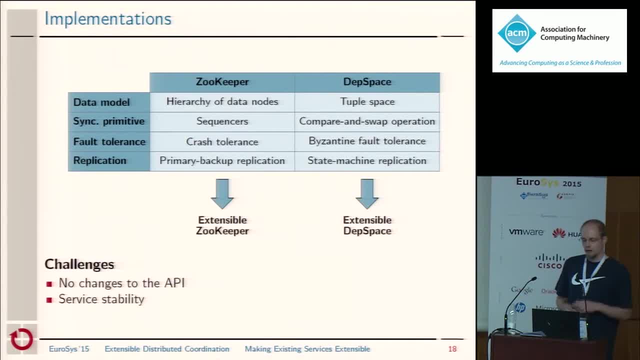 extensible zookeeper and extensible depth space. now, during the implementation work, We basically faced two challenges. the first thing was: we do not did not want to Add new functions to the kernel because it would make it larger. So the kernel should it's- in terms of the set of functions It's provides it should stay the same. 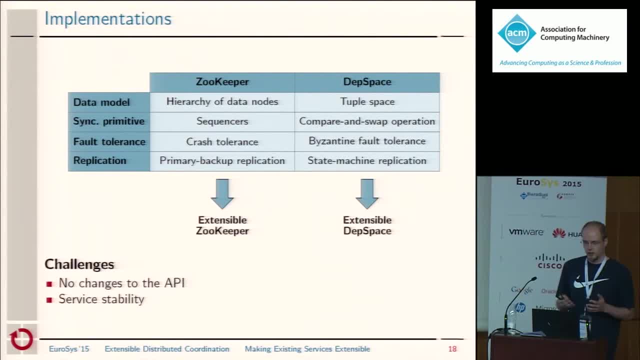 And still provide extensibility. the second challenge was with regard to service stability. We want To limit the damage an extension can do. for example, if an extension is poorly implemented and it crashes at some point, It should not bring down the entire server. So how did we do this in order to make a coordination service extensible? 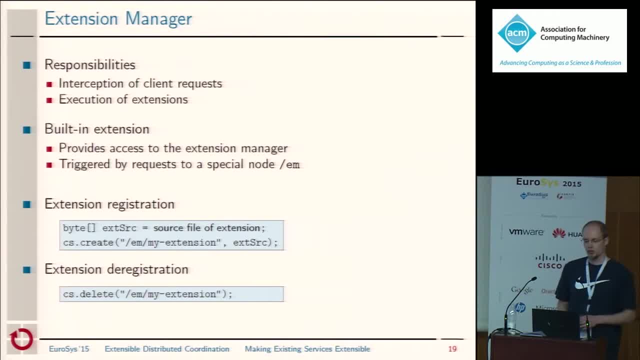 What we do is we introduce a new component, the extension manager, which is responsible for intercepting client requests, checking whether a request Actually triggers an extension or not. If it does not trigger an extension, It is just executed as a regular operation. However, if it triggers an extension, the extension manager is also. 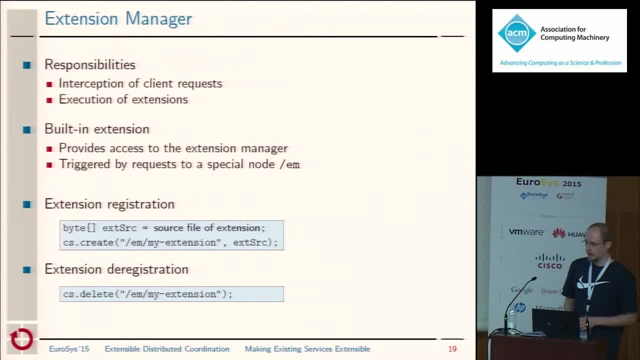 responsible for executing this extension. this extension- now, usually The extension manager- is completely transparent to the client. There's no need for a client to interact with the extension manager. However, there are two exceptions, and these are extension registration and extension deregistration. So for these cases where a client actually needs to communicate with the extension manager, 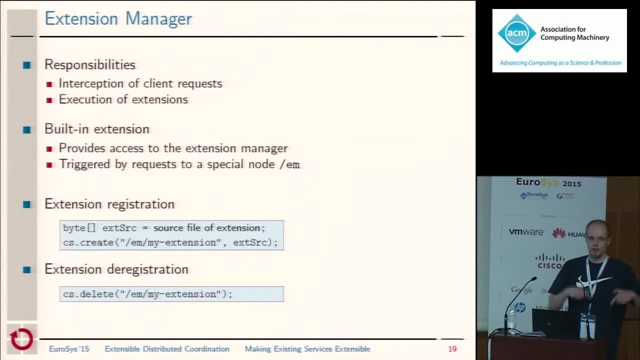 We've created a built-in extension Which is hardwired into the service and which provides a special note in the case of extension zookeeper. This is slash EM, through which a client is able to communicate with the extension manager. So, for extension registration, for example, what the client does is it takes the source file of the extension which contains the code to be executed. 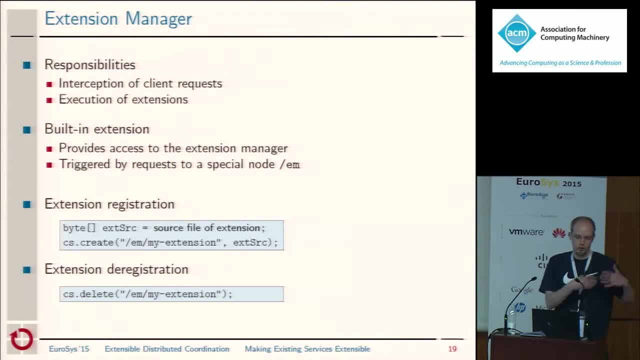 when the extension is triggered, as well as some configuration information on When the extension should actually be triggered. so in the example I showed you, it would say: okay for a node. next, If the get data method is invoked, please trigger this extension. so the client takes the source file and 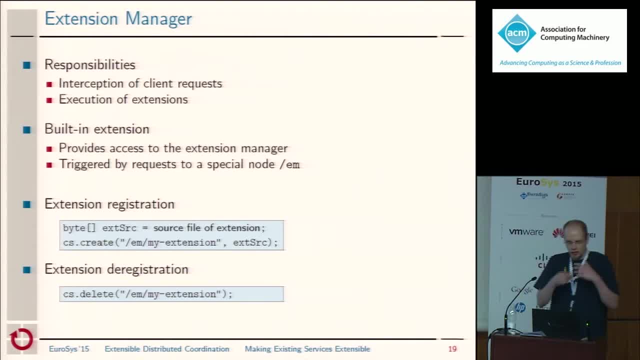 Creates a sub node of this slash EM node on just as a like a regular node. So for the client there is no difference. We don't need a separate method to actually register a register an extension, But just the fact that we create a sub node of the slash EM. 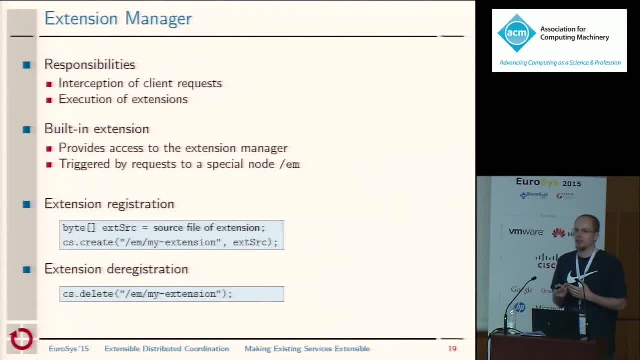 Note. this means that the building extension will be triggered and it will take care of actually actually registering the extension For extension deregistration. basically the same thing, no additional method necessary. all the Client needs to do is to delete the sub node It has created earlier and the building extension will take care of removing the extension from the service. 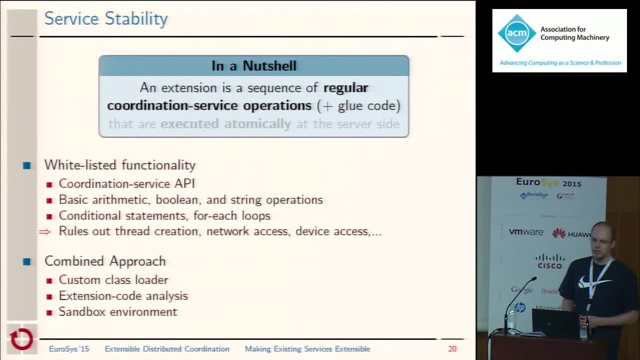 So, with regard to service stability, What we did was we reminded ourselves of our Kind of definition of an extension as a sequence of regular correlation service operations, plus a little bit of glue code and the ideas To enforce that an extension is actually that. so what we did was we took a whitelist approach. 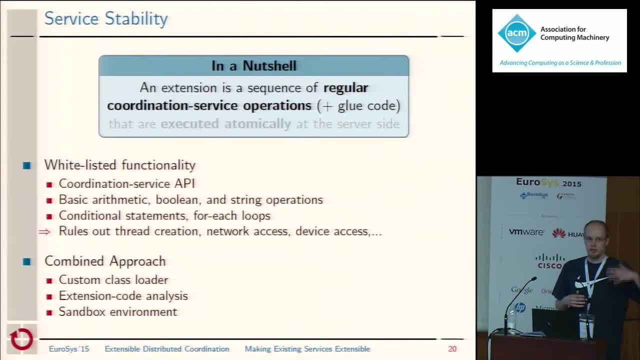 where we just listed some elements an extension may consist of, And Elements which are not on this list are not allowed an extension, So this whitelist contains, of course, the methods that are part of the適合同じр service API. This whitelist contains basic arithmetic boolean string operations. 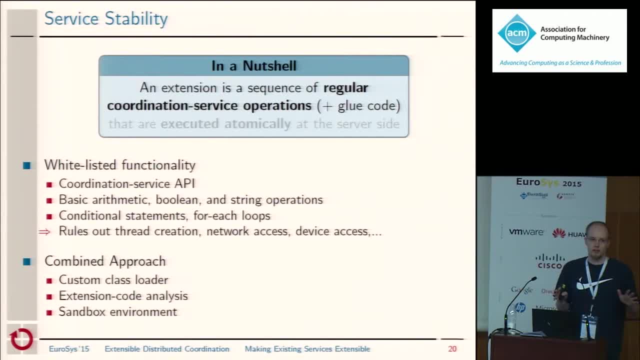 Some conditional statements for each loop and that's basically it. So an extension? There's no need for an extension to create threads. There's no need for an extension to access the network. There's no need for an extension to access an extension to get access to the thread or to create thread or any additional extension to to need an extension setting downtown in another extensive network or to. 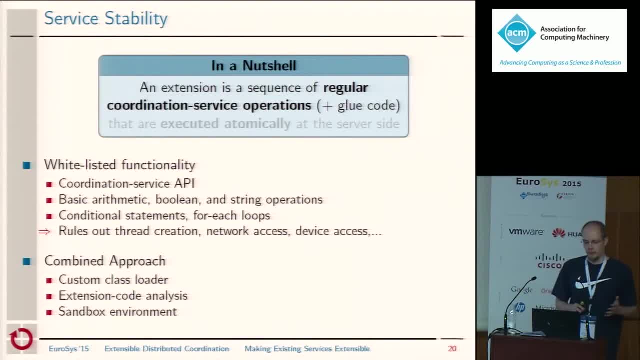 to access devices, so extensions are not allowed to do this, and the way we are currently enforcing this in our prototypes is to use a combined approach which is based on a custom Java class loader, which, for example, ensures that an extension is only allowed to load and use the classes that are on the 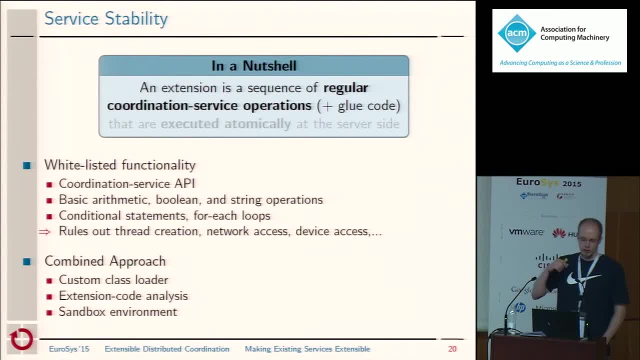 whitelist. This, for example, prevents an extension from just calling system exit and shutting down the entire Java virtual machine. There are some things we do not catch with the class loader. For that we have extension code analysis prior to the extension registration and during the extension execution. the 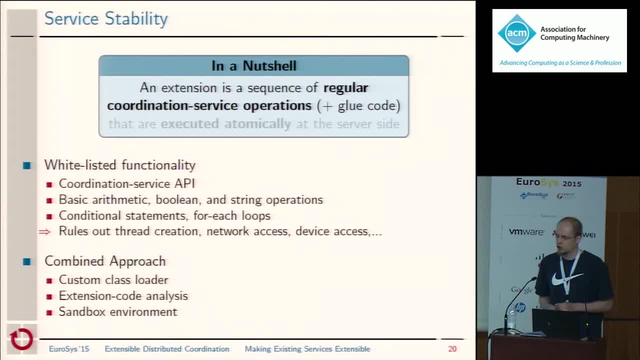 extension is executed inside a sandbox environment which ensures that if the extension crashes, this crash is dealt with and it does not take down the entire service. Plus, the extension sandbox environment also allows us to monitor what an extension does to the service state and probably deny the extension access if it does something we don't want it to do. 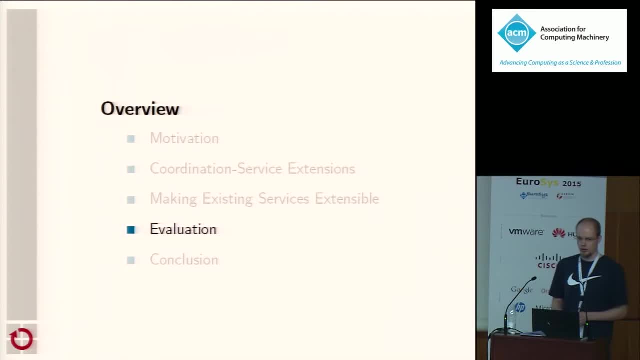 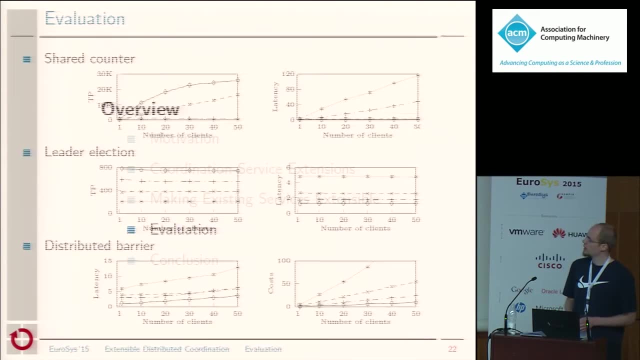 So we've seen earlier that an extension is a good means to efficiently improve the distributed queue. We've implemented additional coordination mechanisms: a shared counter support for leader election and a distributed barrier. I won't have time to get into all the details. 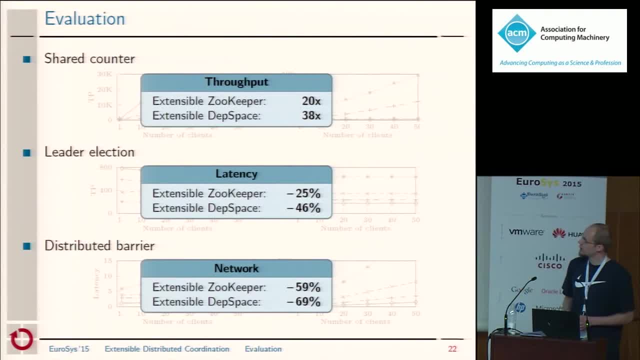 so, therefore, just a summary of the evaluation results. The shared counter suffered from the same problem as the distributed queue. Also, it has problems with contention, which allowed the extension-based version to improve the throughput of the shared counter even more, in this case by 20x and 38x in ZooKeeper and DepthSpace respectively. 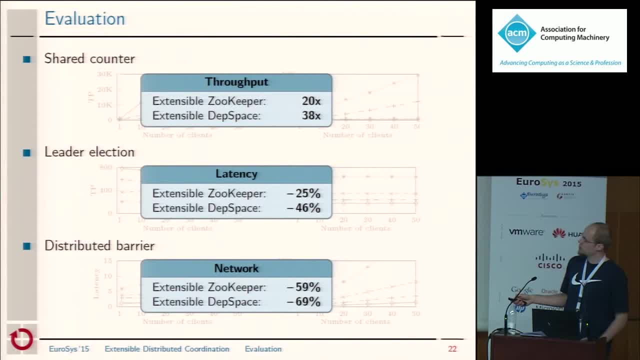 In contrast, the other two coordination mechanisms- leader election and distributed barrier- did not suffer from concurrency issues. Here the benefit of the extension is to reduce the number of remote calls a client needs to do something. This reduction in remote calls, for example, leads to a lower latency for leader election of a fourth in ZooKeeper. 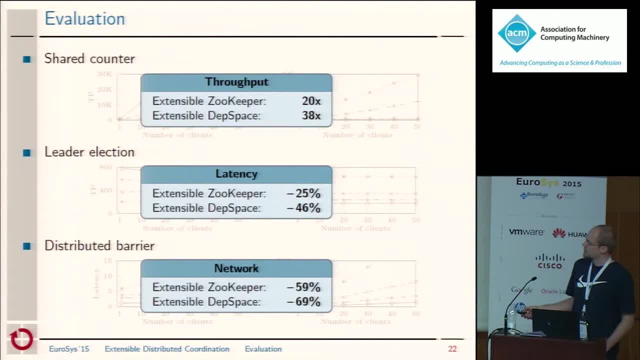 and almost half in DepthSpace, as well as savings in the amount of data a client needs to send to the network. In this way, the distribution barrier is reduced by about two-thirds of the amount of data a client needs to send to the coordination service for the distributed barrier. 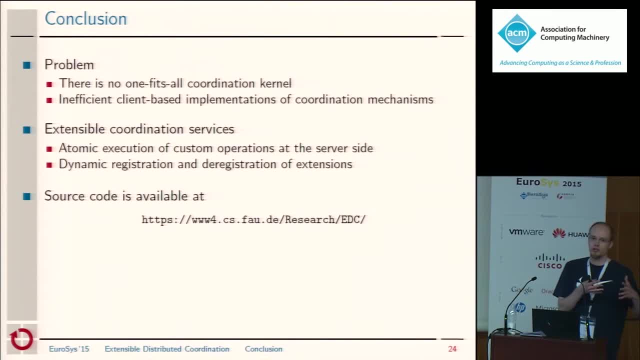 So, in conclusion, having a small coordination kernel is a good idea, but the problem is that, as there is no one-fits-all coordination kernel, as clients have to implement more complex abstractions themselves, there is the potential of the danger of ending up with 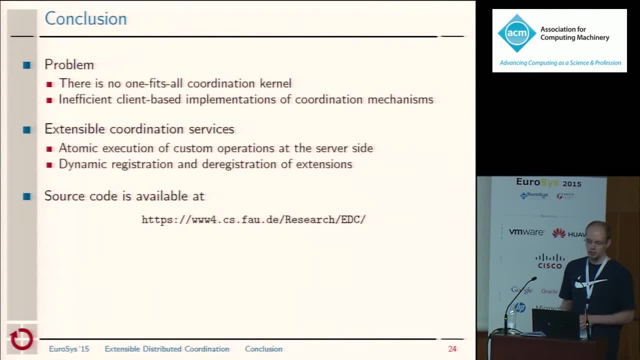 very inefficient implementations. Our approach to deal with this problem is to make coordination services extensible, which means a client is able to write custom operations, register them at the servers. they're executed automically there and after the client is done, the extensions will be removed from the servers. 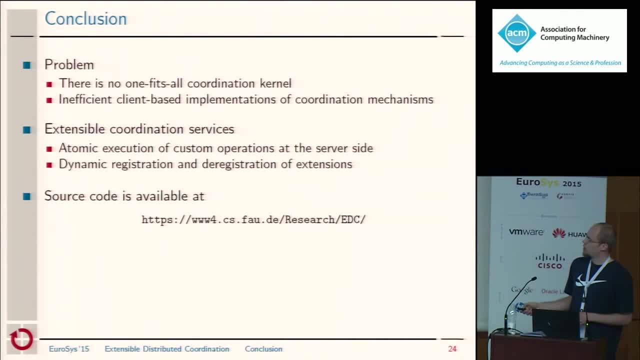 So if you're interested in, please take a look at our website. The code for both extensible ZooKeeper well as extensible depth space is available. That's the end of my talk. Thank you very much. I'm happy to take questions. 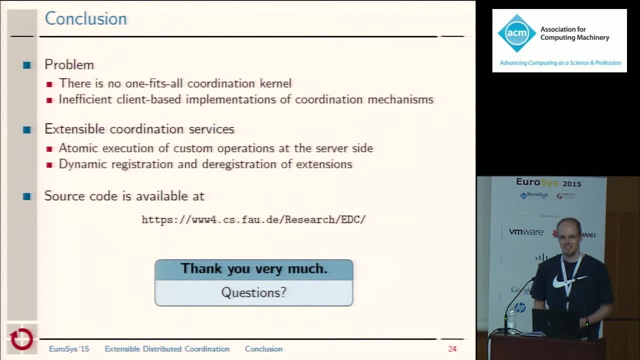 Many people leaving. One of the very nice features in ZooKeeper is the ability to set watches on data. Is that something you support in one way or the other, or is it just not necessary in the model that you propose? I'm sorry, did you ask about the watches? 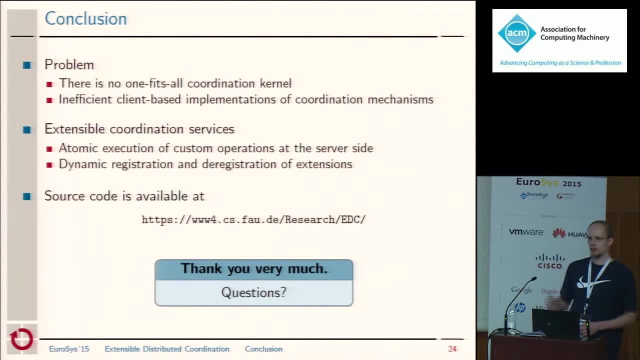 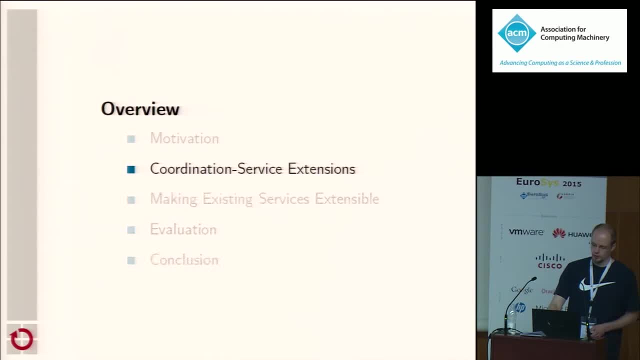 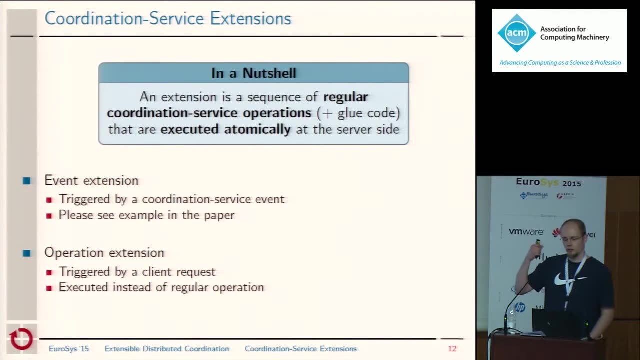 Yeah Yeah, The watches is an example of an event extension. So, as I said earlier, we have two types of extensions: event extensions and operation extensions. In ZooKeeper, an event extension would allow you to customize what a watch can do or when a watch will be triggered, And this, for example, is a good 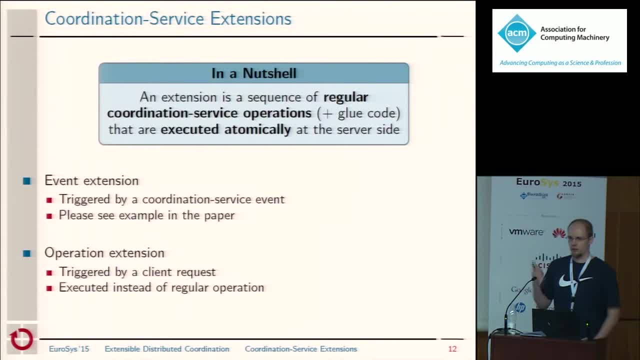 means to improve the legal action coordination mechanisms. Thanks John Wilkes at Google. If I understand this right, it's basically a software engineering argument that by providing an extensible service framework platform thingy you can make it easier for people to put together new implementations of their particular coordination framework.